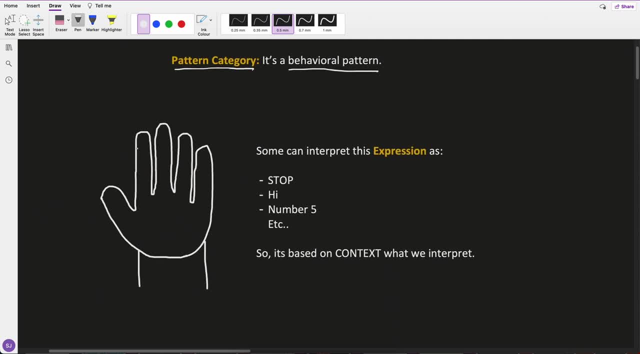 to behavioral pattern. Okay, so now let's understand. first what does interpreter pattern means? Consider: this is a hand sign. What do you interpret out of it? So either you can interpret it as a stop or somebody saying hi to you, or it might be denotion of number five. or you can say: 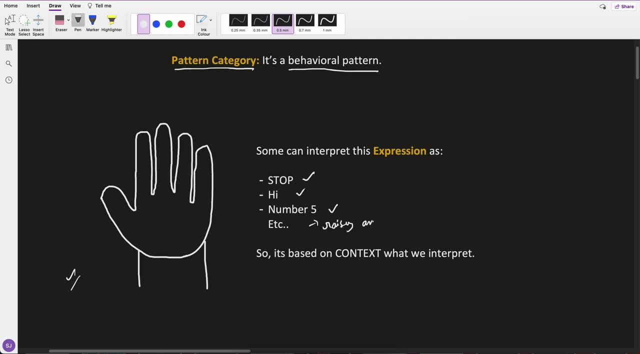 that it might be like a raising a hand. So this sign can be interpreted in different ways. So it depends upon context, In what context we are providing or what is the context, and based on that context we can say that, hey, it means stop. For example, context I give you that it's a traffic signal or something. then the 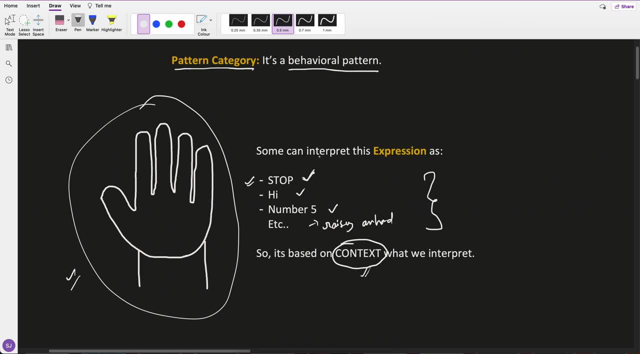 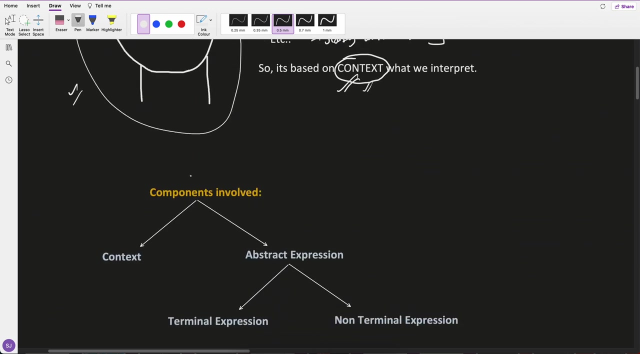 stop sign. there might be like a stop somewhere. So what I'm trying to say is that interpreter means the way you interpret the expression, the way you Understand any particular language, Right. So interpreted design pattern is a way through which you can understand any particular language, Right? Okay, So what are the components involved in it? 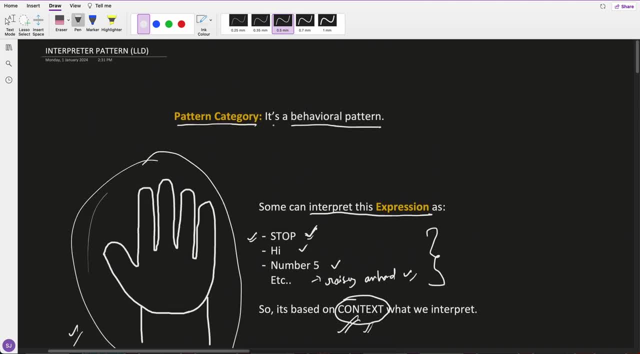 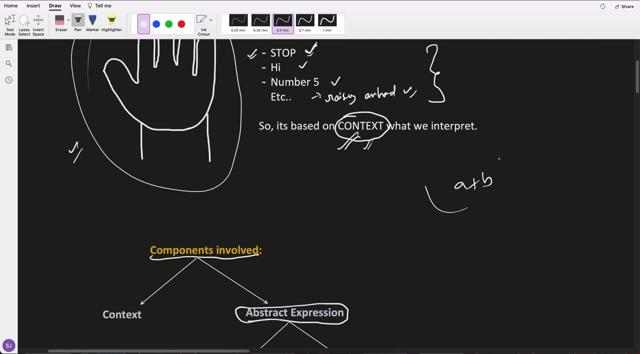 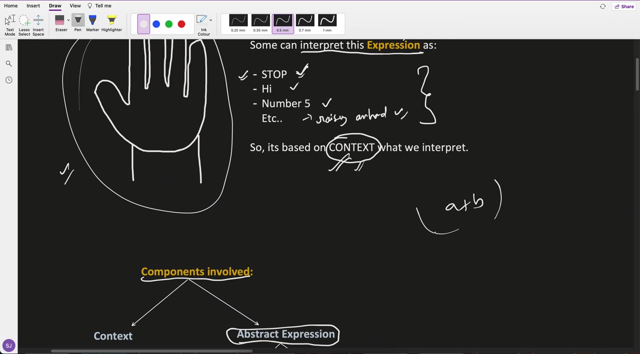 Abstract expression. So now, when so interpreted pattern is specifically for understanding the expression. So expression could be, let's say, A plus B. This is an expression Right. So any expression you can interpret based upon the context which we will provide, Right. So this is also. 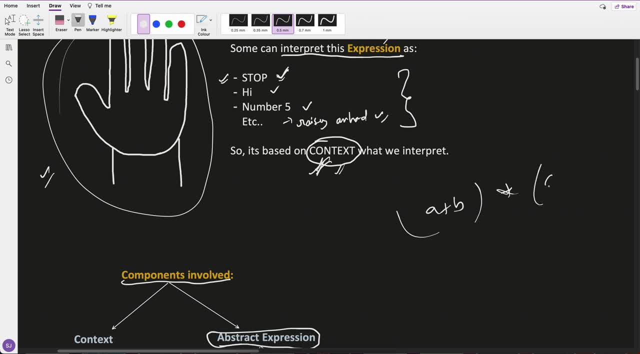 considered as an expression Right, So into C, into D, This is also an expression Right. So interpret design pattern can be used to understand this expression. or you can say that to compute this expression, but based on a particular context, we will provide to it Right What it understand with this. 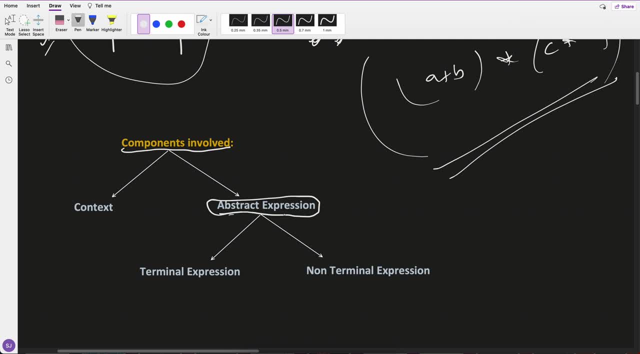 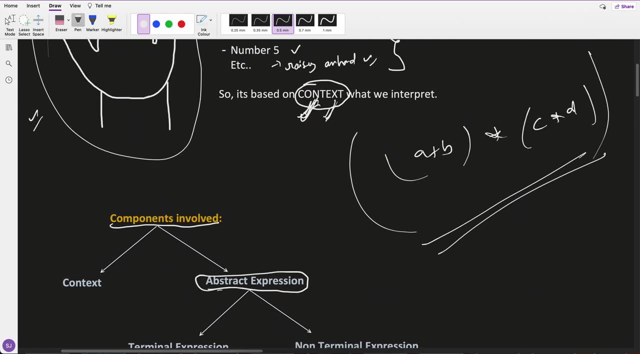 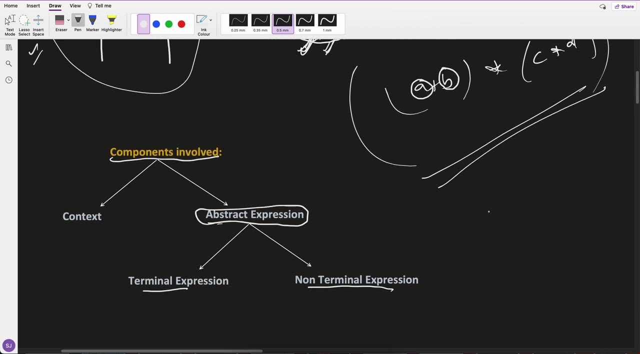 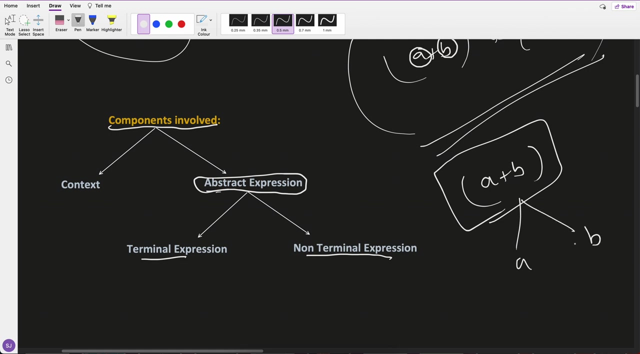 So we have an abstract expression, and abstract expression has two things: Terminal expression and non-terminal expression. So here, if you see that these are, terminal expression means you cannot further divide it. But this A plus B, This is a non-terminal expression. This can further be divided into A and this can be divided into B. 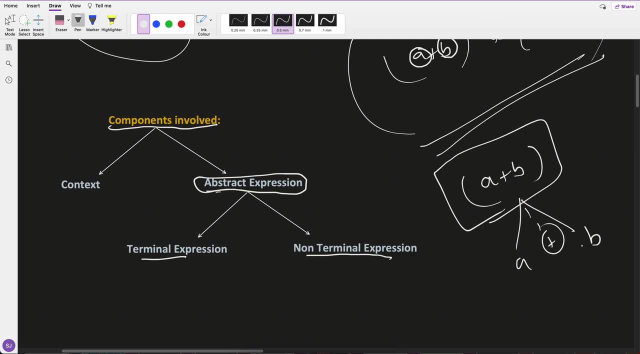 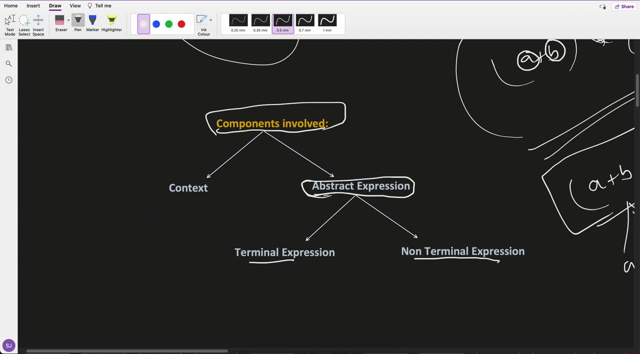 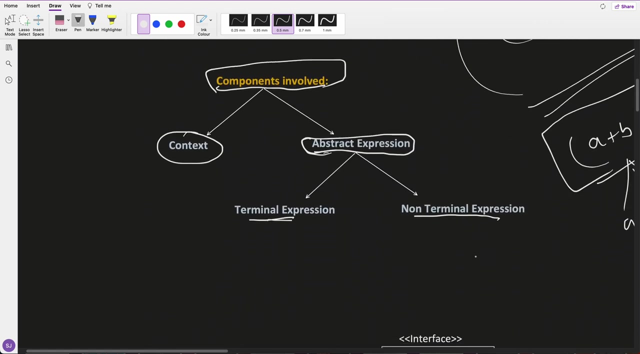 And this is like plus, Do the plus of it. Okay. So abstract expression. So what are the components involved? So, components involved is one is abstract expression And another is context. Abstract expression can be have terminal or non-terminal. Okay. So we will see an example and you will get fully clarified with it. This is the UML diagram of it. 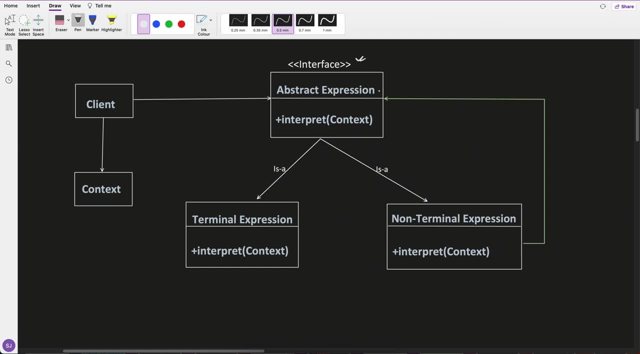 Right. So here, if you see that we have an interface- Abstract expression- There we have a method called interpret and we pass the context to it. I told you Right What we had in the interpret design pattern: we have to interpret an expression using a context. 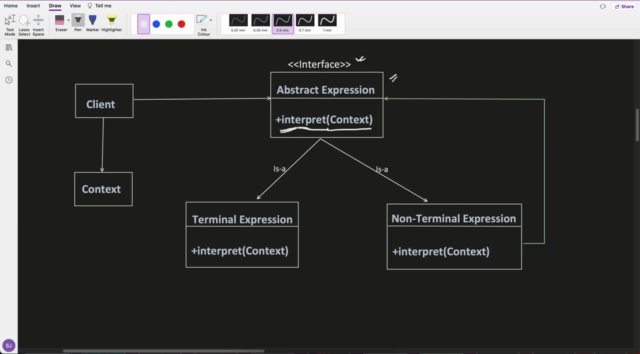 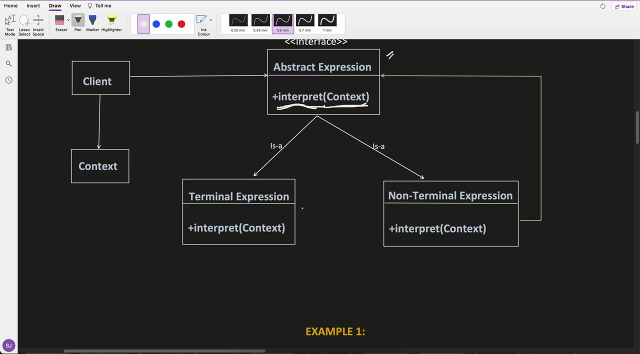 Right. So abstract expression has one method interpreted and it received one context. Now there are two type of abstract expression can be terminal expression, Right, And the same method it has to implement. non-terminal expression And the same method it has to implement. And then there is a client. 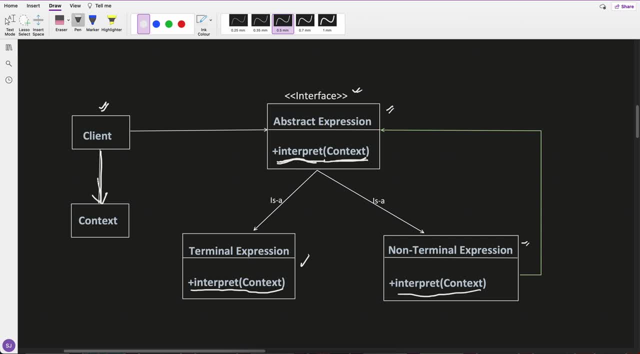 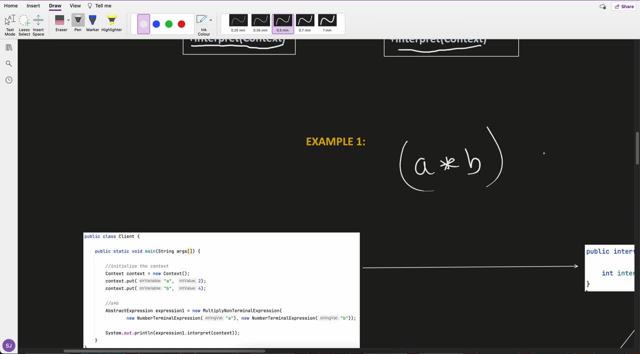 Okay. So we'll see an example where let's say that I want to do A into B- Okay. So we'll see an example where let's say that I want to do A into B- Okay. So we'll see an example where let's say that I want to do A into B. This is one expression. 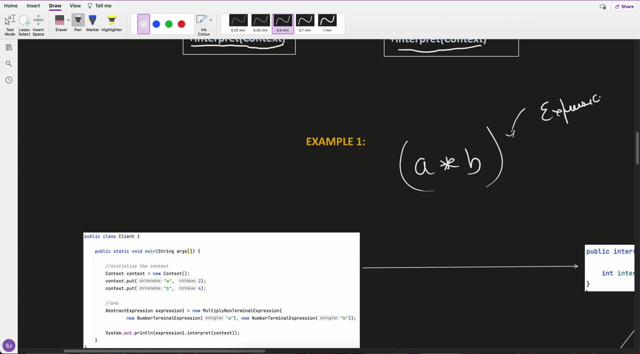 Okay. So we'll see an example where let's say that I want to do A into B. This is one expression. Okay, So we'll see an example where let's say that I want to do A into B. This is one expression. This is one expression. Okay. So we'll see an example where let's say that I want to do A into B. This is one expression. This is one expression, Okay. So we'll see an example where let's say that I want to do A into B. This is one expression. This is one expression. Now, what should be the output? 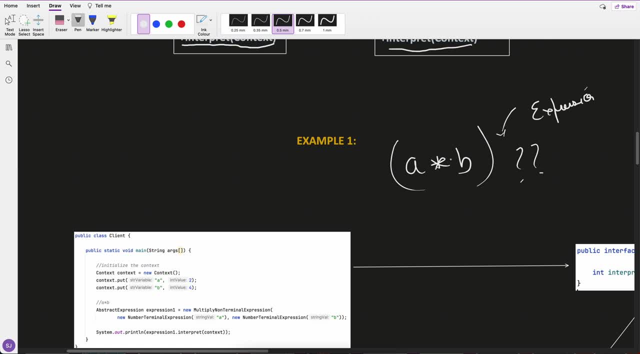 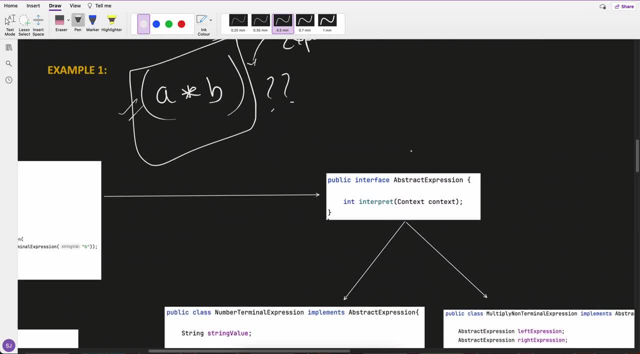 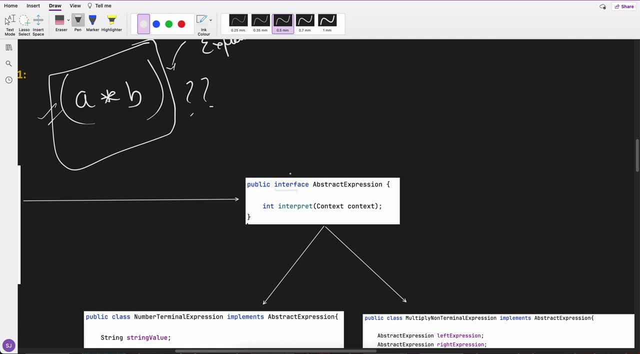 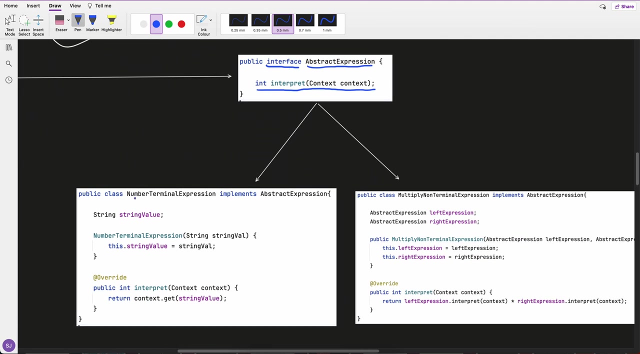 Okay, So now here we'll say that. let's see one by one component which we have in the UML right. First is abstract expression. So I have created one interface, I created one here, interface, abstract expression and the abstract method like interpret context. Okay, Then there is one number terminal expression. So this is a terminal expression, which implies that the 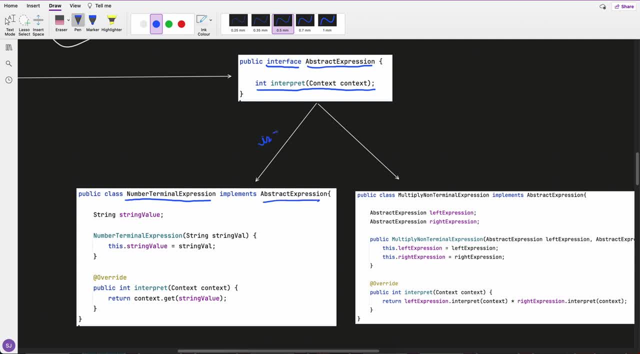 string will implement this abstract expression. So this is a relationship. Okay, So I'm getting one string value and using this constructor to assign this string value, right? So this is a method which it has to implement. So, whatever the context it will get for this string value, it will using that context to get the data for it. 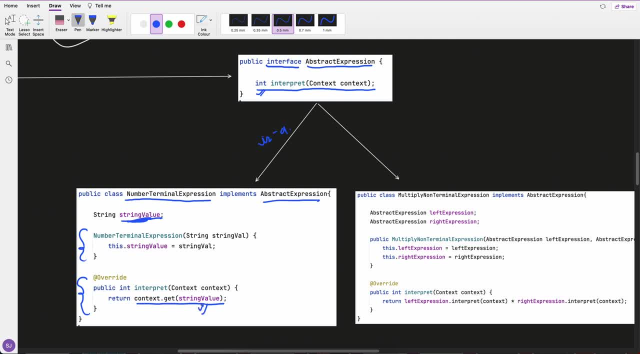 Hey, context, this is the data I am getting. Tell me what I have to do with it Now. context will give it right What it interpret. This is a terminal. I am doing Now in a non-terminal expression. I have given the name multiply, non-terminal expression. So A into B. we wanted to do right. So this full is a non-terminal, This individual. 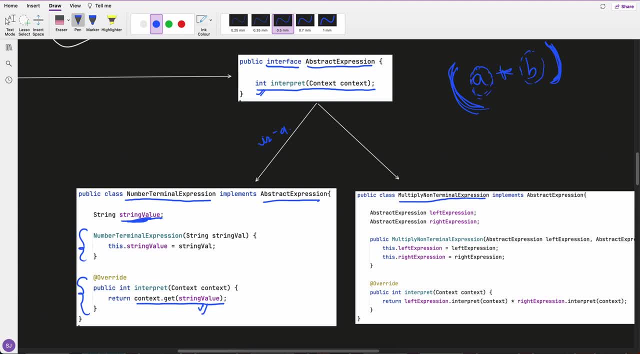 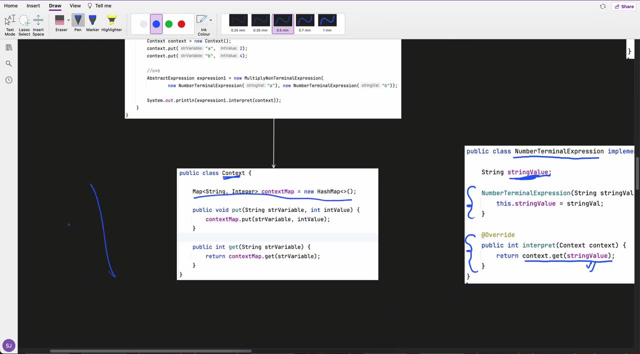 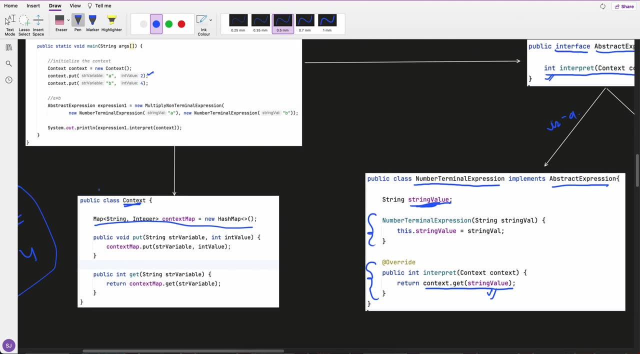 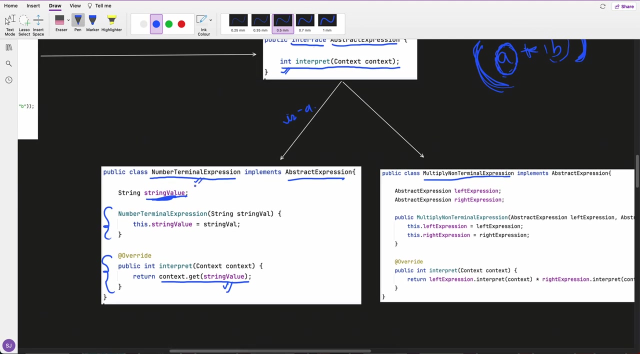 is a terminal. So for A in the context here, if you see the context in the context I, I created a map, map of what A considered A as two, B as four, So map is this. So now, when this particular A goes to the terminal expression, right. So for this, A, contextget A. So it. 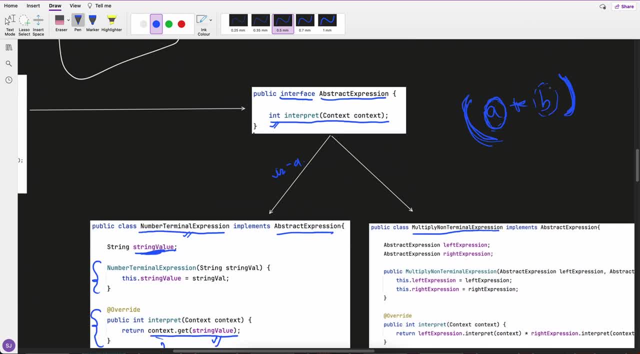 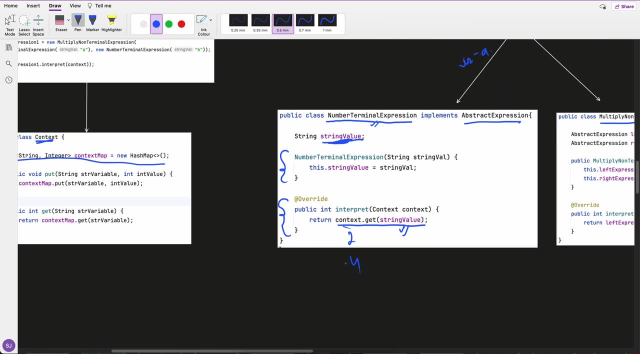 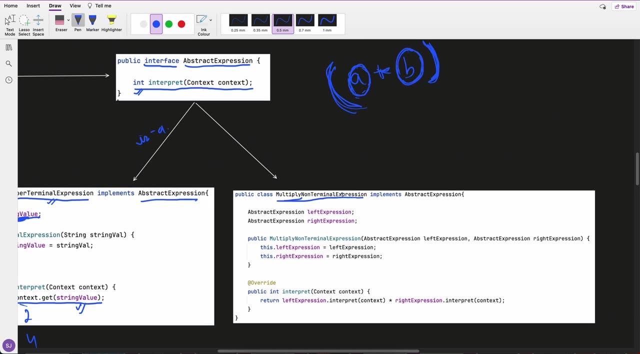 So it will return two from here. So when it get B- so context dot get B, so B would be four- it will return four out of this. Okay, now, in the multiply non-terminal expression, what it will do is we have left expression. 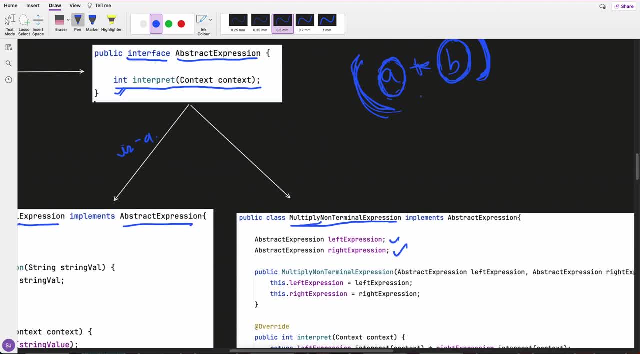 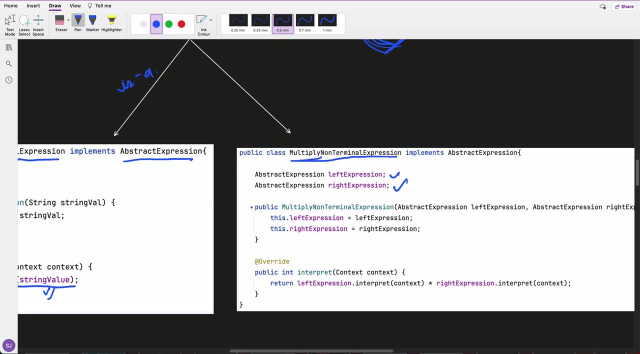 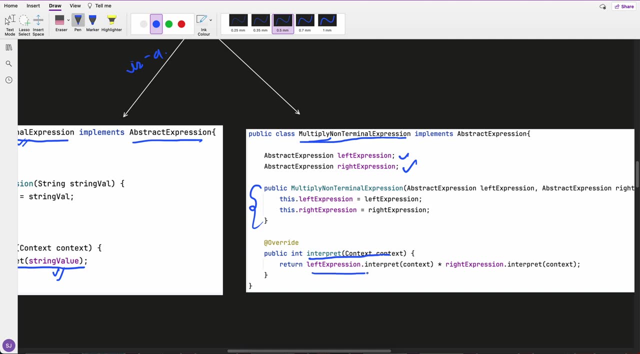 and right expression, right Left expression and right expression. So in this multiplication we have left expression, right expression, right. So this is just a constructor to assign the left and right and in the it's interpret method we have to call the left expression. 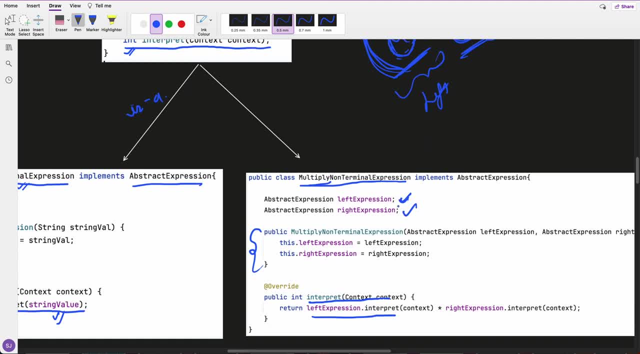 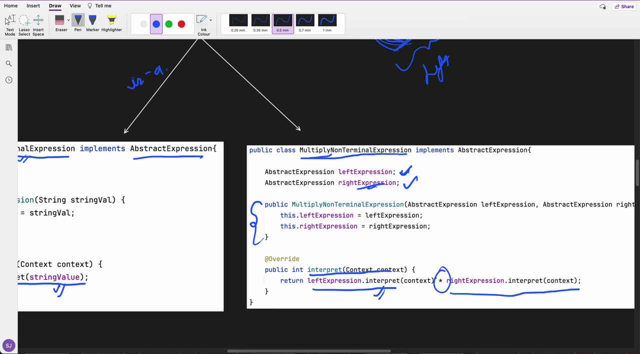 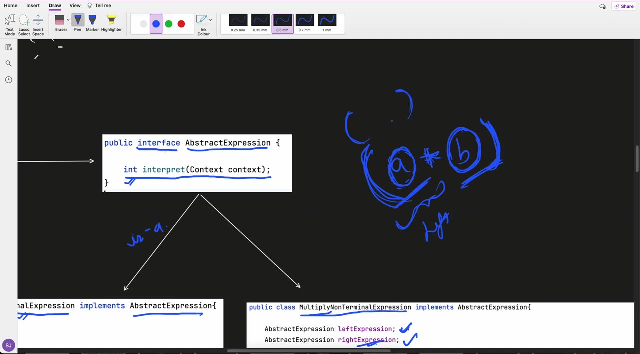 whatever the left expression would be, we have to call it interpret method and whatever the right expression would be, we have to call it it's interpret method and we have to multiply it right? So maybe if left expression is further a non-terminal expression, 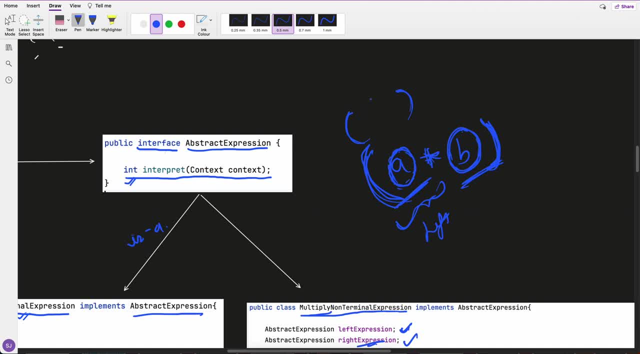 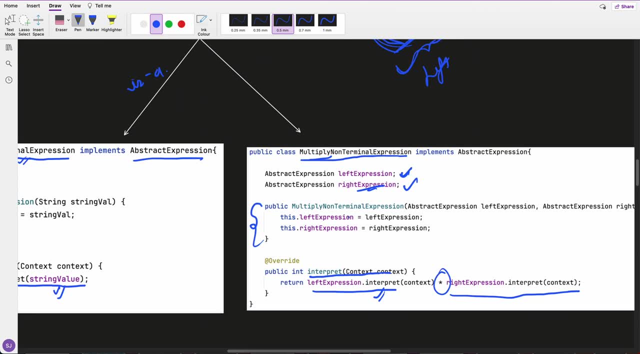 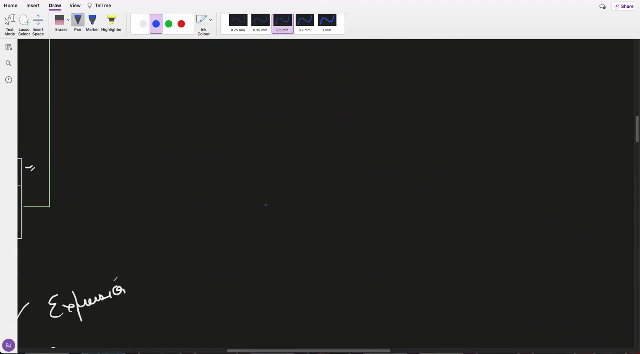 you can say that it will kind of recursion. then it will again call the multiply non-terminal right. Might be So, but what I am trying to say here is in the non-terminal expression right. We are again calling this like here: 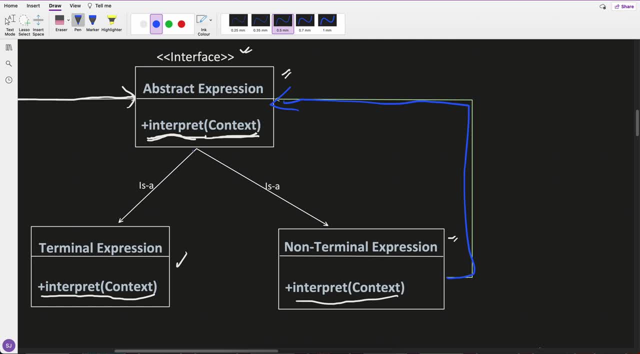 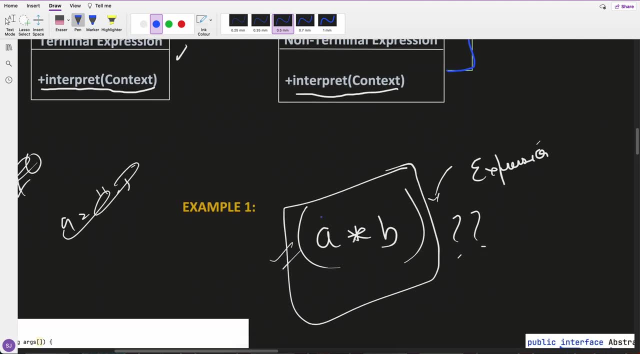 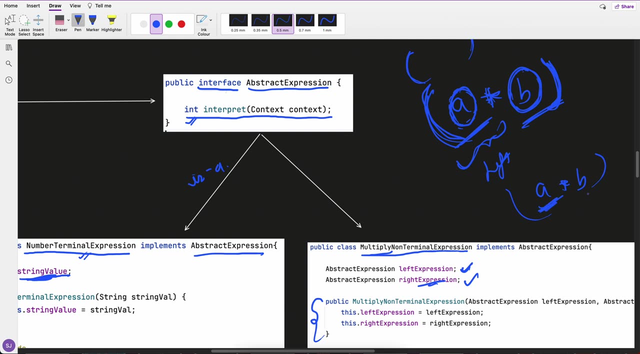 The interpret method right And either it will go ahead and call the terminal or again go and call non-terminal. So by far it will go ahead path. it will go ahead path, depending upon the expression. but for this A into B. 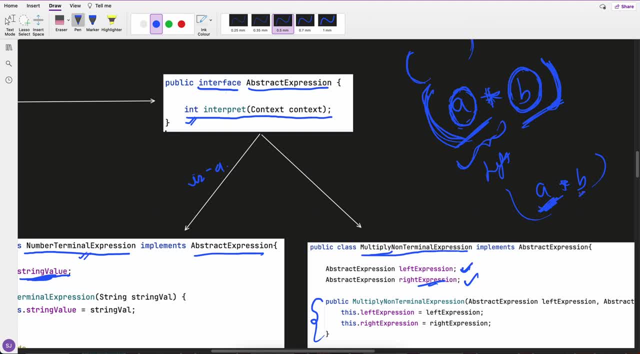 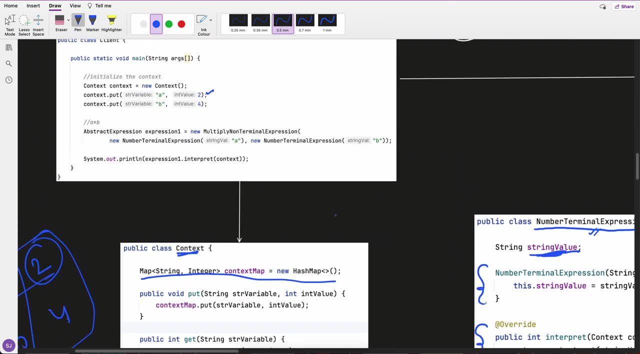 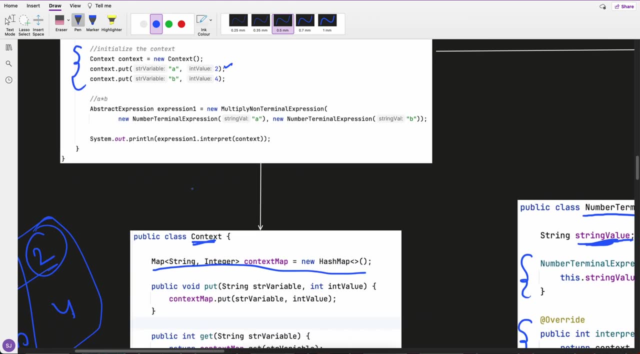 the left is your non-terminal and right is also non-terminal. we have provided Okay. And if you see the client now here, if you see in the client what I'm doing in the client, I am first setting the context. So I created a context object. 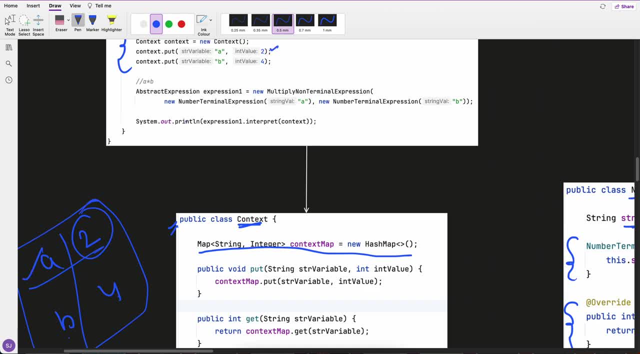 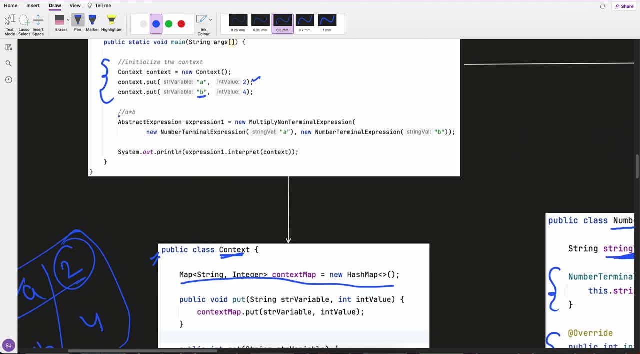 I created the context object. now in the map I have put this two-way typo in contextEurope: state values A. I have assigned 2 and B. I have assigned 4 in the map. right, these are the string. now I am trying to interpret this expression. so what I am doing is new multiple non-terminal expression. so 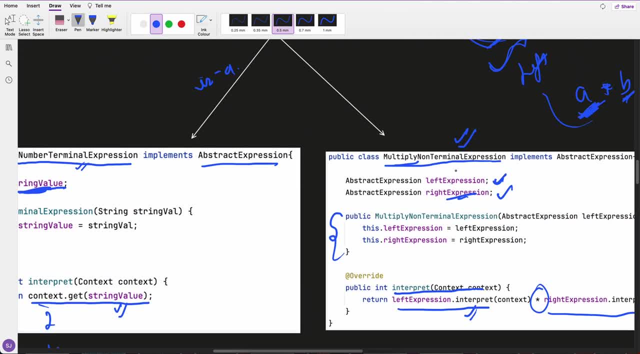 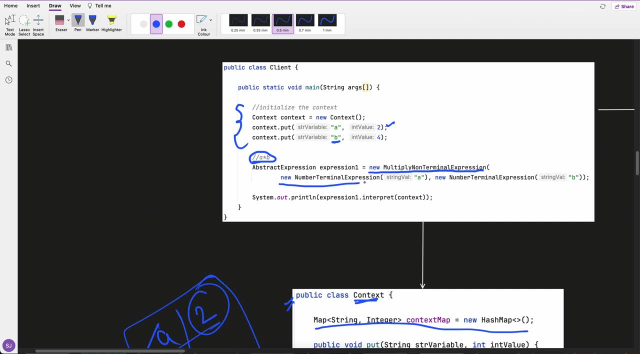 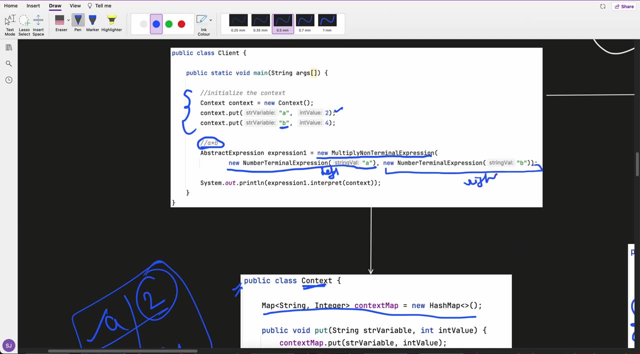 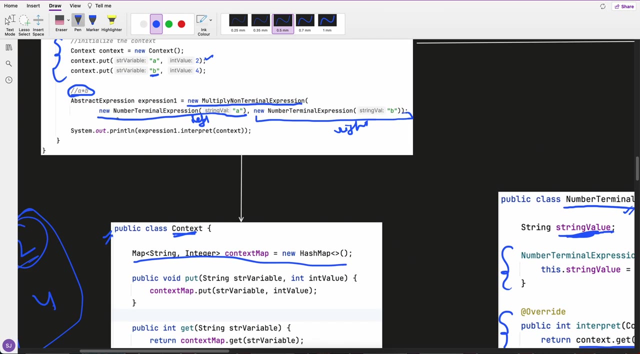 I am creating this object, its object. now, this object, it accept two expression: left, and right, right. so I am giving this left, this is my left, and here it is right, right. so in the left, what I have provided in the left expression, I have provided number, terminal expression right. so it's. 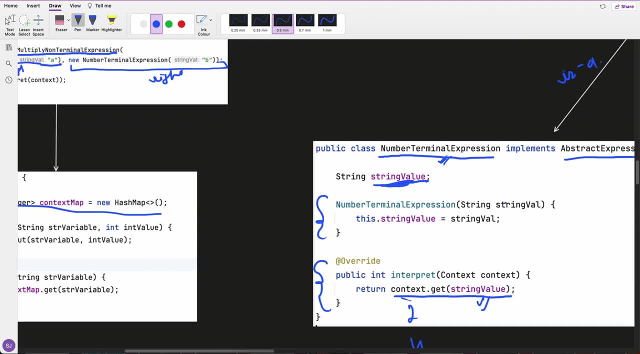 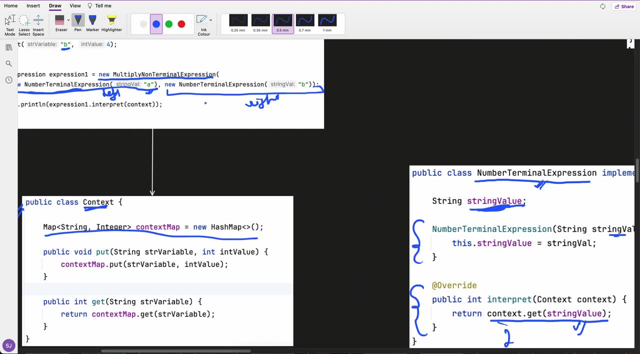 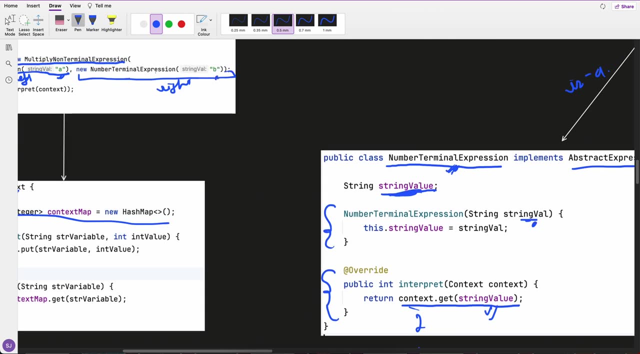 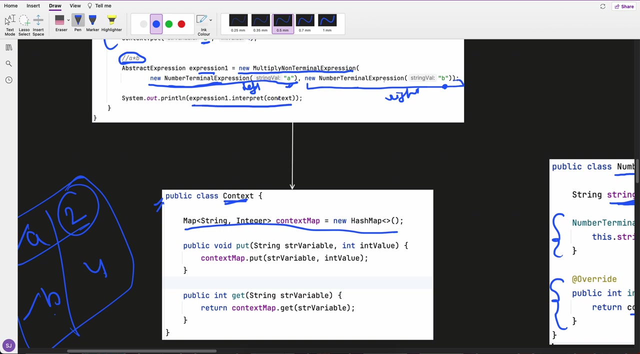 a number terminal expression I provided. and what is the string value I have provided here, a in the right expression. what I have provided, again a number terminal expression, and what is the string value I have provided in the constructor, be, okay, and whatever the expression I have called the interpret and pass the context. now what will? 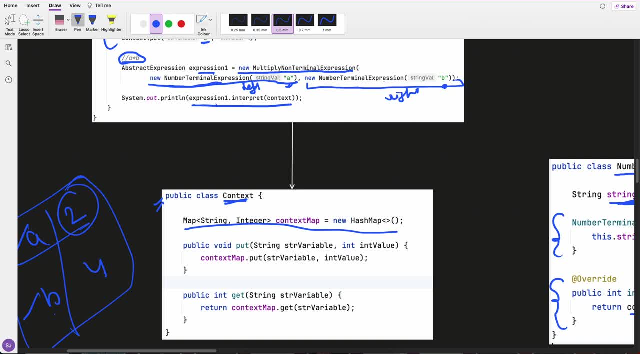 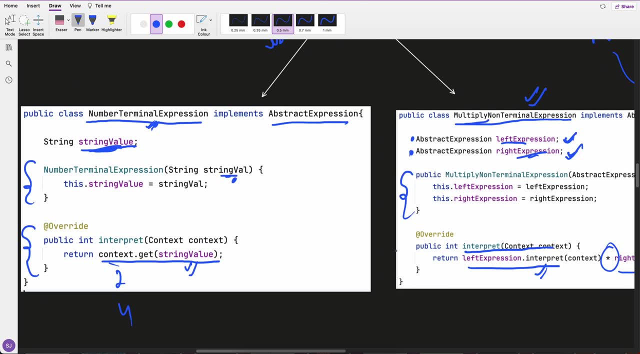 happen is this expression dot interpret. so what it will call is multiply non terminal context. it will call this method right: this two are all equal and this one two are not named. it is useless. okay, let us go ahead and now system is going to integrate two different and it is scared of. 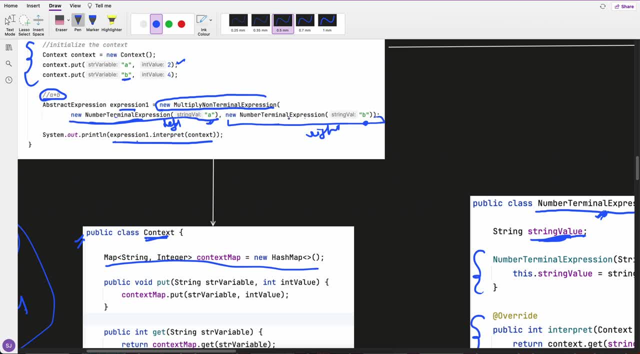 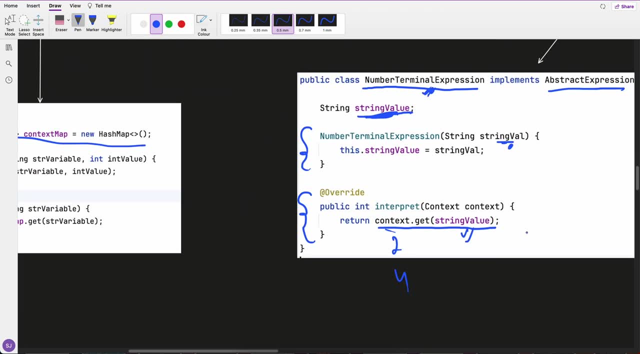 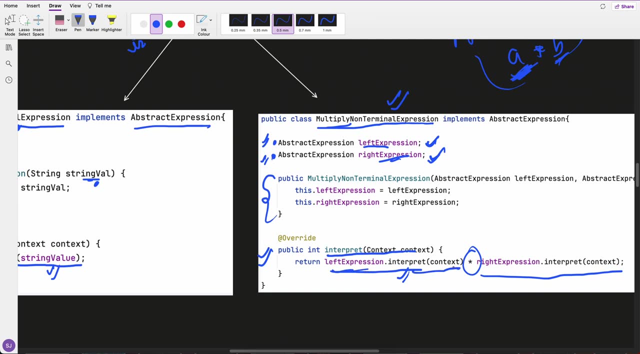 already set with this number terminal and with a number terminal with value b, okay, and I have called the interpret and pass the context. So here what I am doing is I am calling the left expression, dot interpret, and passing forward the context into right expression, dot interpret this one. 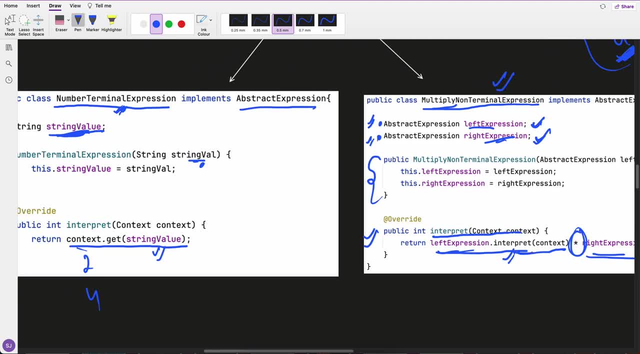 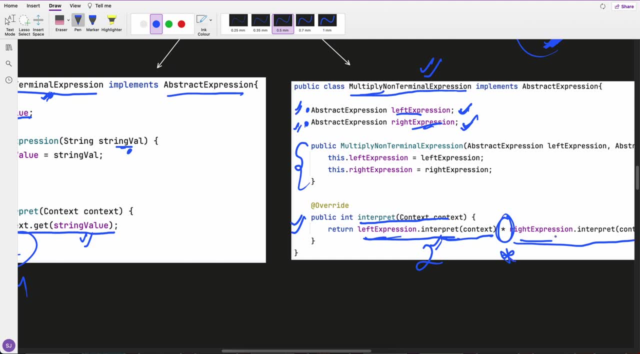 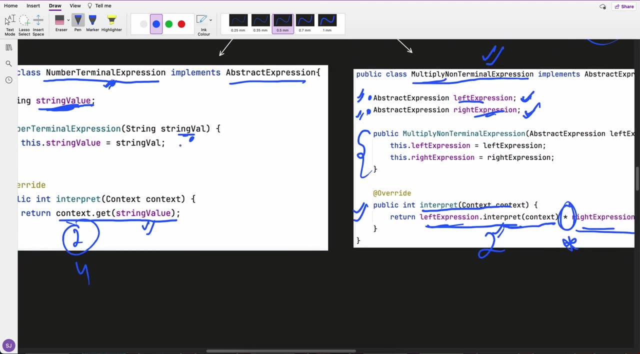 So left expression was number terminal right and so it was a. So for a it will return two, so two into. for right expression was also your number one, right and b. So it will call this interpret method with the value b and for b it will return four. 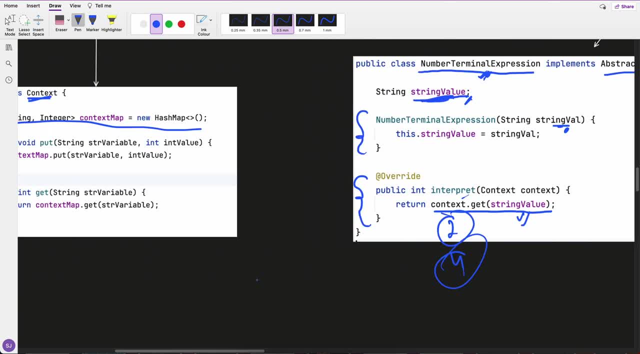 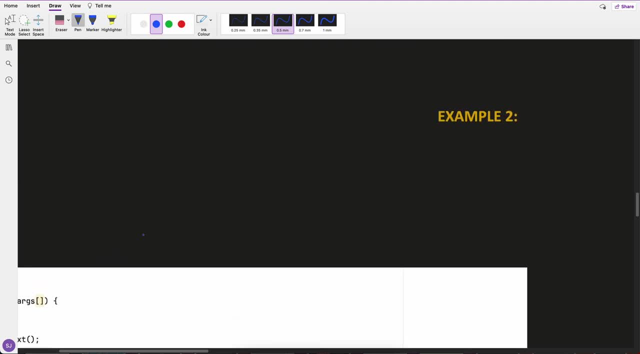 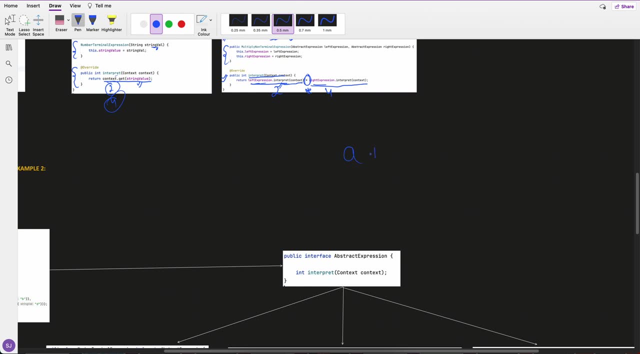 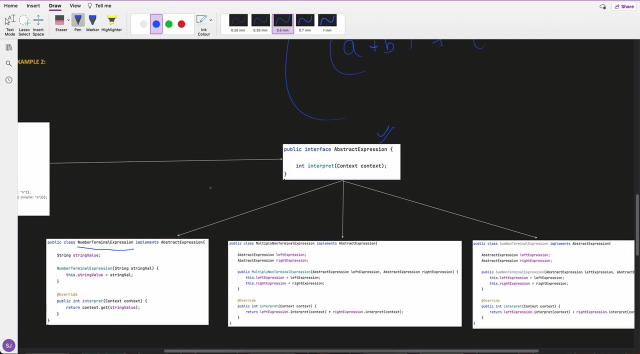 so two into four. ultimately this will return your eight. So you got it. So we can Solve harder expressions also the same. So let's say I want to solve a into b plus c into d, right? So one way is that here in the abstract expression I have a terminal expression number like all. 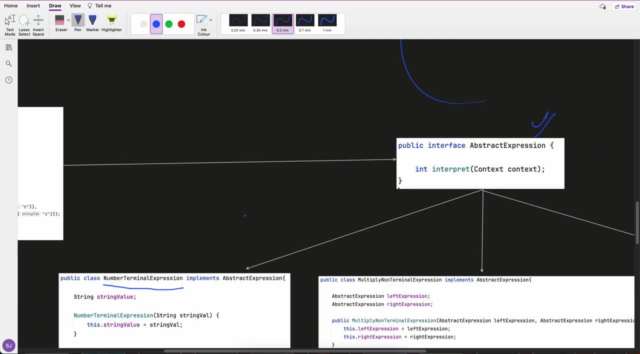 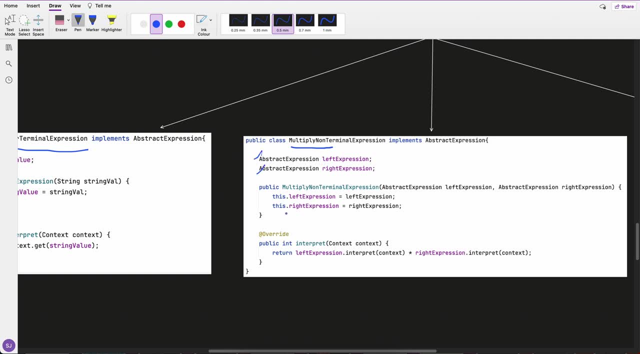 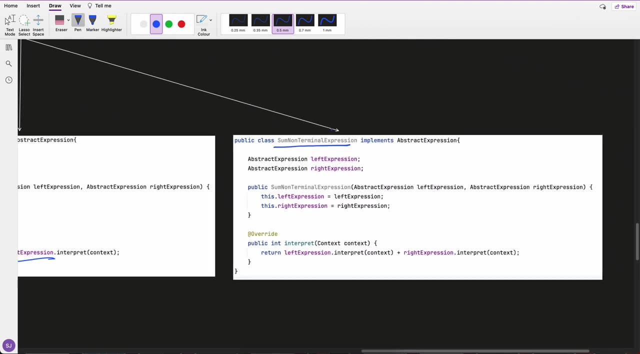 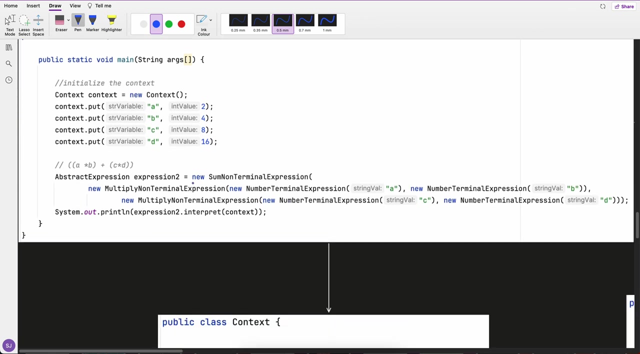 these are terminal. Then I have one Multiply expression, right, So, which has left and right, and ultimately it multiplies those. Then I created some expression which again has left, right and actually do plus yet if you see that first in the sum, So a into b plus c into d. 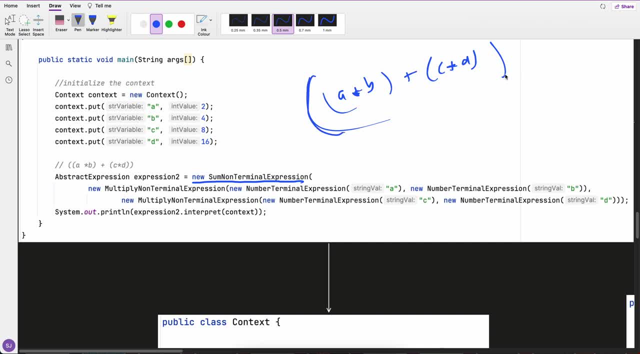 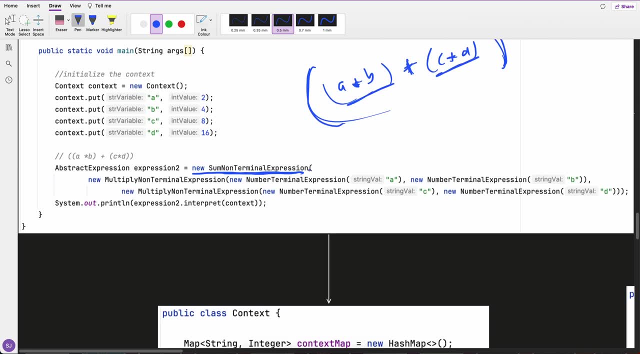 We want to do this, So first we have to do some This plus. So Sum of what Two multiplications. So this is the first Multiply non terminal expression. This is the second non terminal expression, Right And for each. 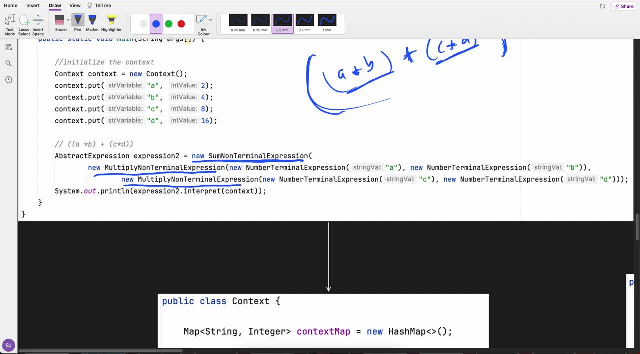 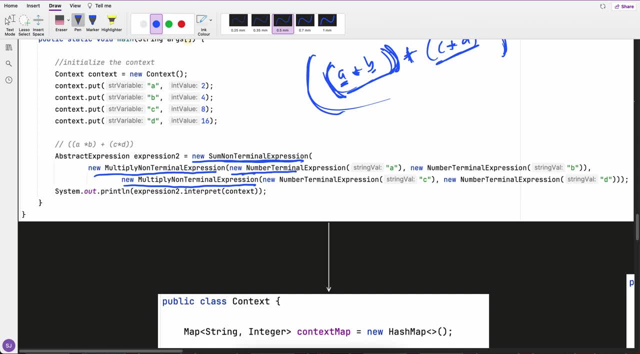 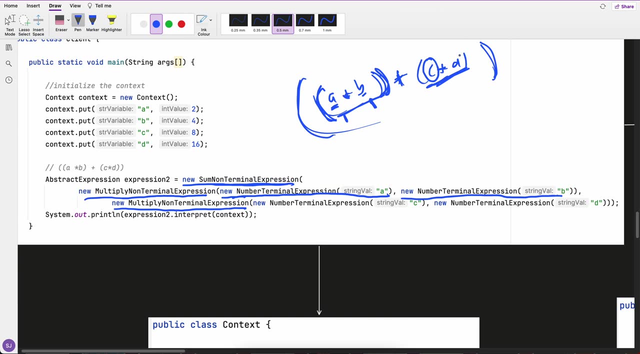 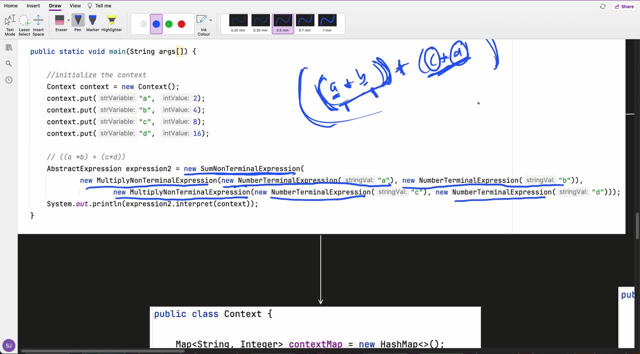 The way Your tough expression would be Right. So We have created this expression. Now we are Wanted to interpret this expression, So we are calling he interpret this expression expression and pass the context and the context map. I have put a considered a as 2, b as 4. 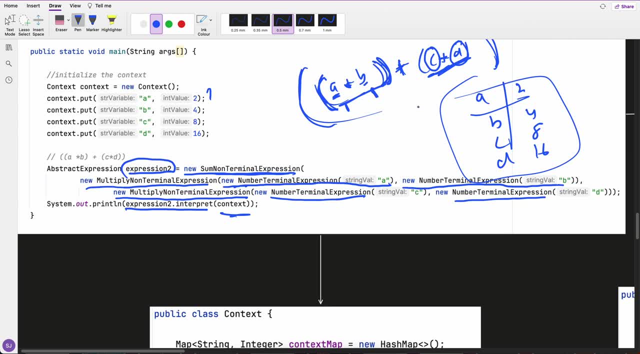 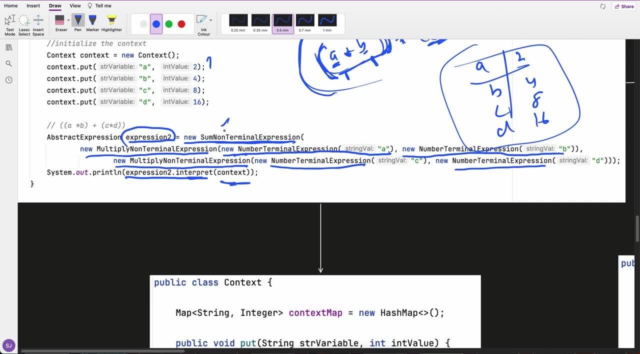 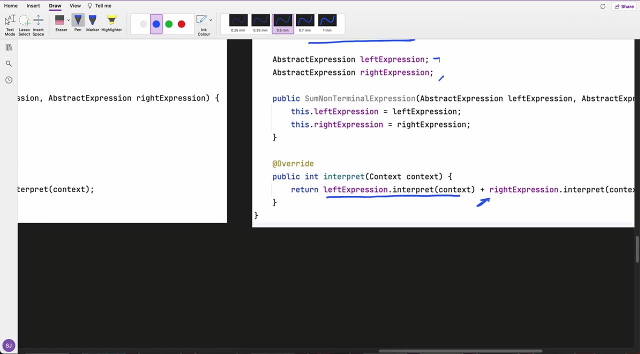 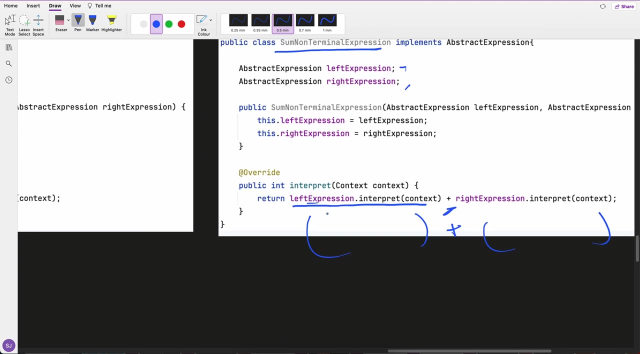 c as 8 and d as 16 right, and now I am passing this expression. I wanted to interpret it and do the context. so, first expression: it goes to the sum. so it will goes to the sum. it will try to do that. hey, expression plus right, and it's right. so left one is right, multiply one. 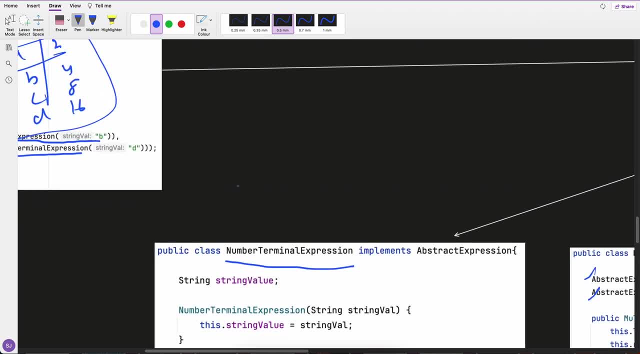 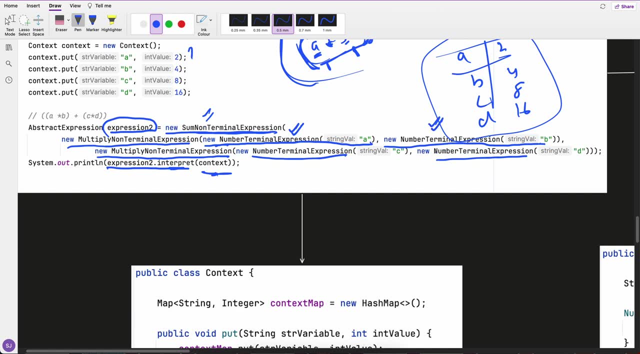 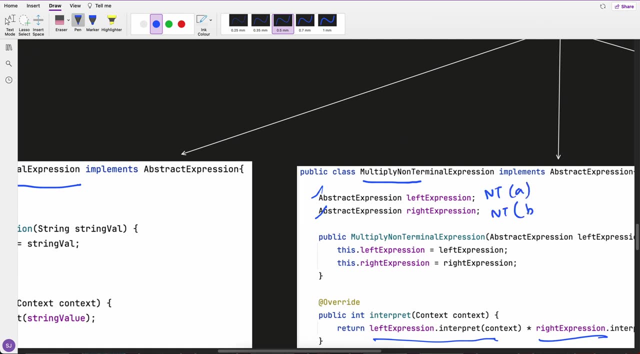 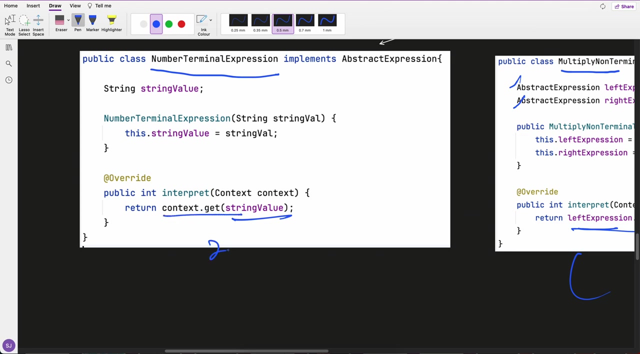 so it will call the multiply this one. it will call the multiply with this two number terminal and a and b number terminal b. so here we have number terminal with a number terminal with b right, So it's left expression. This expression will call number terminal with a, so it will return to two and two number. 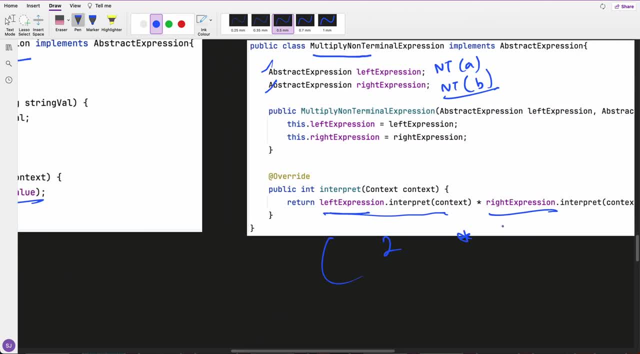 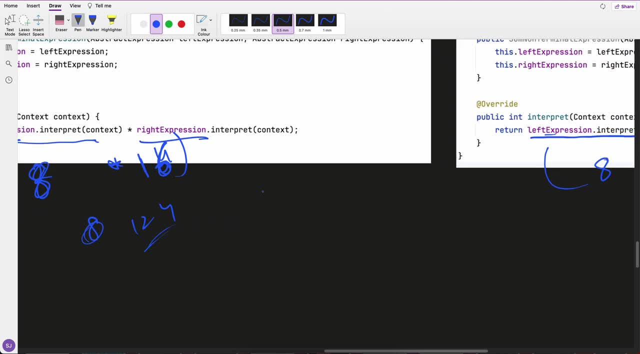 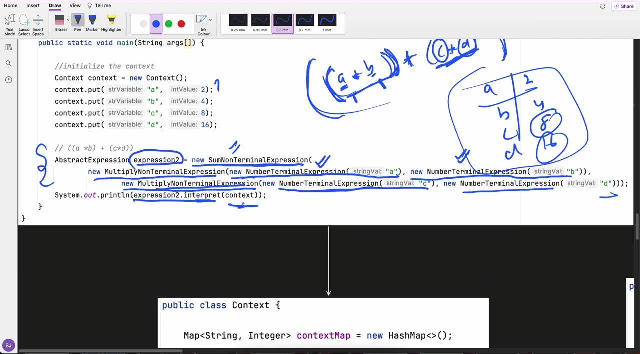 terminal b. so b is your four, so it will return eight. so it's left would get eight. I think you got right the crux, how it is working. So we are computing the expression or interpreting the expression based on the context. you can further optimize it. 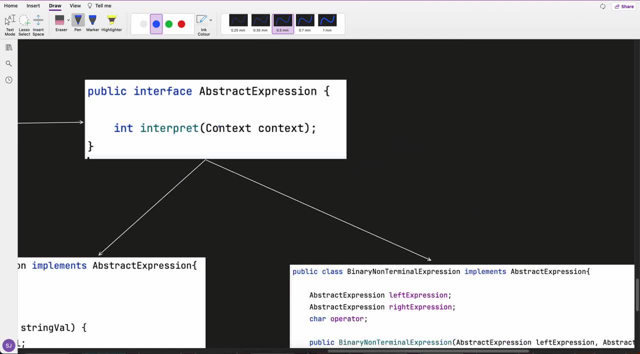 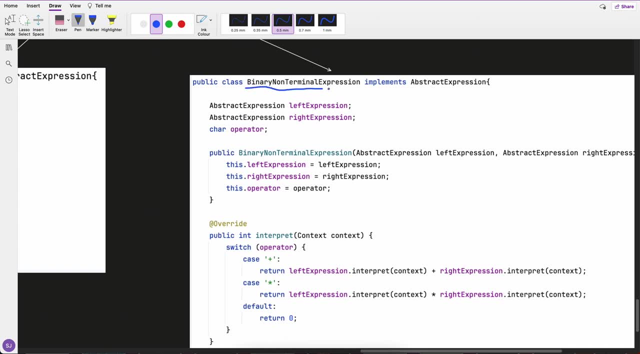 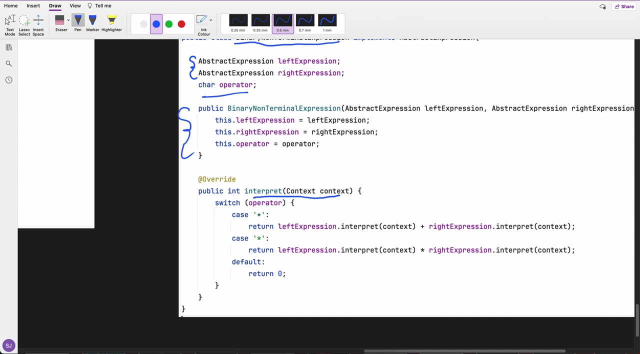 By we let's say that I have further optimize it. instead of creating multipliers, some subtract different, different classes- I have created one class called binary terminal expression, left and right expression and also receiving the operator right, and in the constructor I will receive this and in the interpreter based upon the switch operator, if you are. 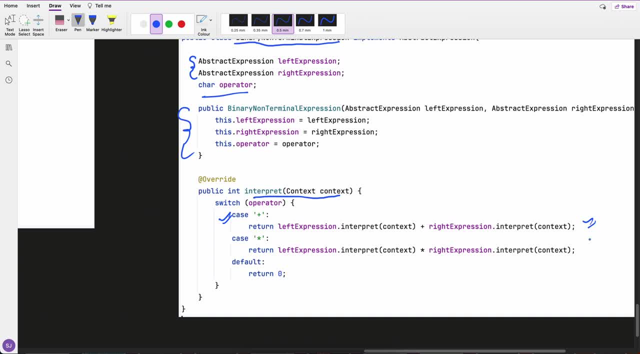 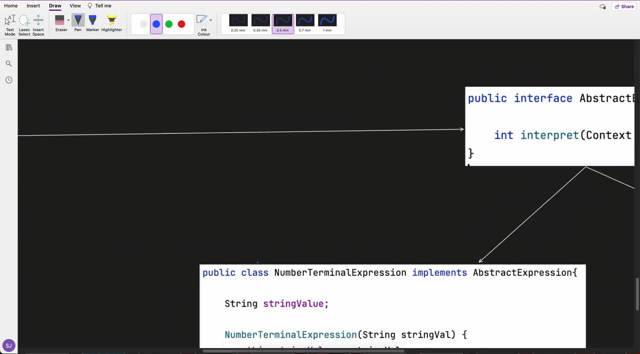 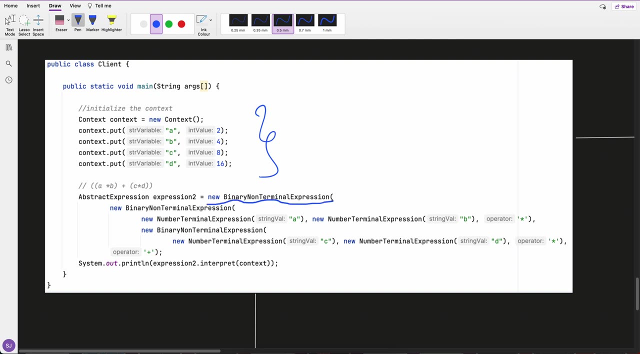 doing plus, do this. If you are doing multiply, run this Okay, Otherwise return zero. let's say I am supporting only two now, here in here. this is the same context which I build up now. I am creating binary terminal expression, right, non terminal expression. I am passing first again a non terminal expression and inside a non terminal.